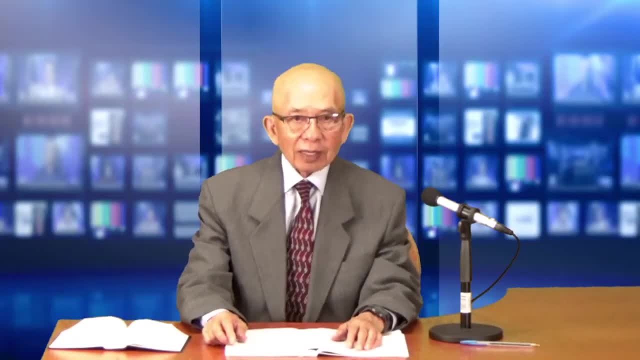 So now, first of all, we know that using the purple, the color purple robe, so it's for those who has money, who are the wealthy, okay, Remember that, only the wealthy that be able to afford to use the color purple, the purple robe, okay. 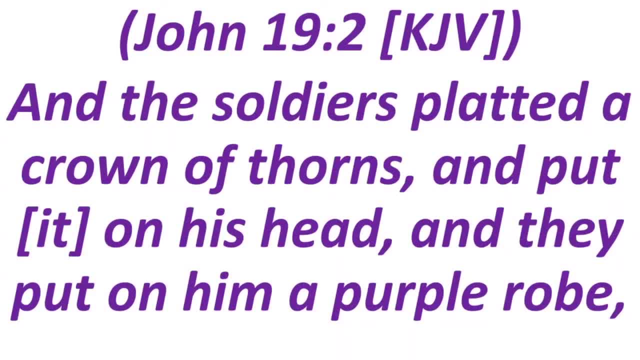 So let's see next scripture. Our next scripture is John 19, 2.. It said: and the soldiers plaited a crown of thorns and put it on his head. And he said: and the soldiers plaited a crown of thorns and put it on his head. 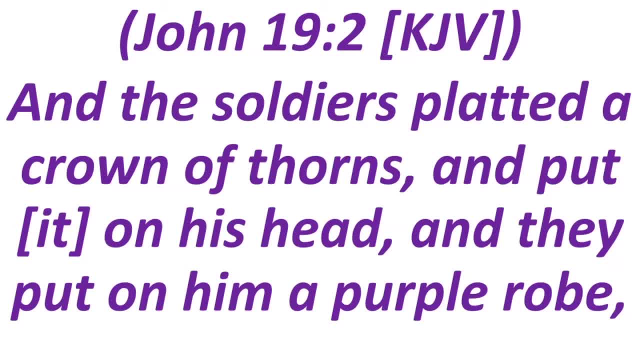 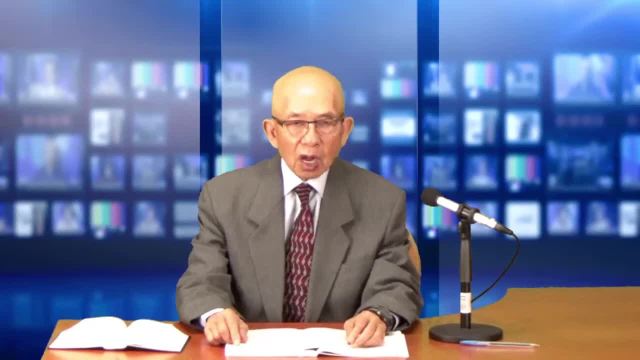 And they put on him a purple robe. So this is. we know that the situation is that Jesus was arrested And for those soldiers who arrested Jesus, they want to mock Jesus because you know from what Jesus claimed? Jesus claimed to be the king of the Jews. 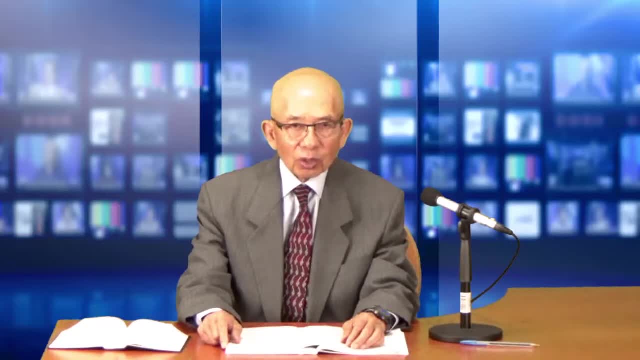 So they want to mock Jesus and want to make fun of him. So they using not the real crown, using the thorn to make the crown and put on his head, So just to mock him And also put the color, the purple color, robe. 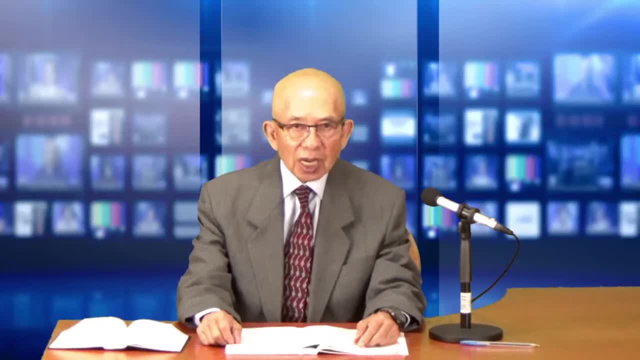 It represents the robe for the king. So if Jesus claimed himself to be the king of the Jews, so he should have the purple robe. So now we have two Bible texts to support that the purple color of the robe is for the wealthy and for the king. 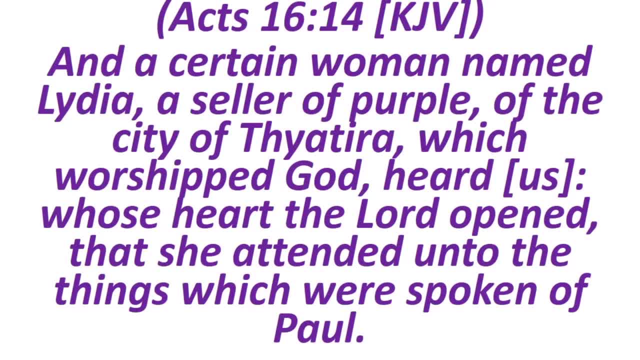 Okay, let's see the next one. The next one is in Acts 16,, 14.. And a certain woman named Lydia, A sailor of purple of the city of Thyatira, which worshiped God, heard us whose heart the Lord opened.